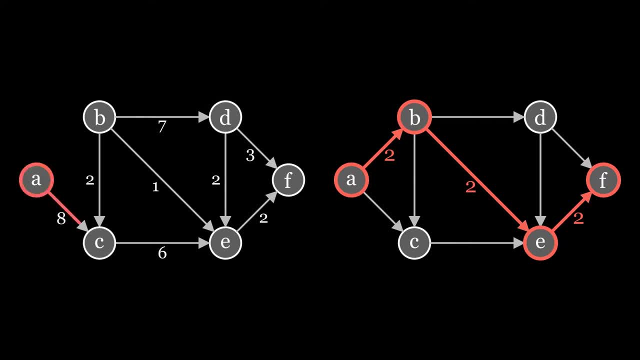 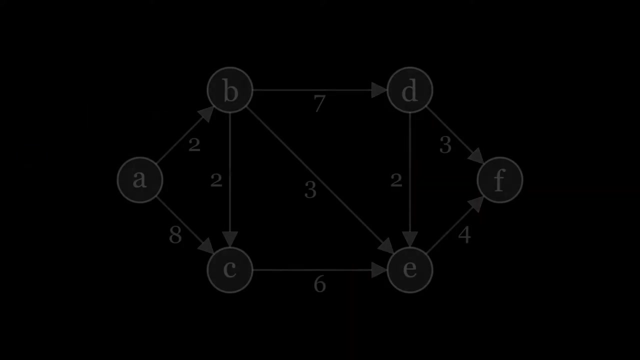 Now we consider a new path, find the bottleneck and add the new flow to the graph on the right. Once again we compute the residual graph. At this point we realize that there are no more paths available. The flow we got is 4, but this is not the maximum flow possible. 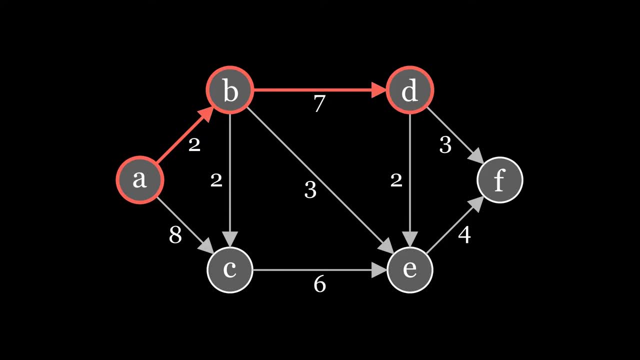 This was caused by an unlucky choice of paths. Here we can see that by choosing different paths we can get the maximum flow for this network, which is 6, given by the sum of the two selected paths. The idea behind the 4-Fulkerson algorithm is to avoid this problem by adding backward edges to the 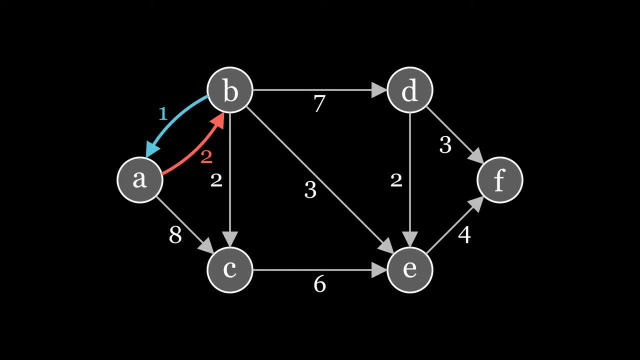 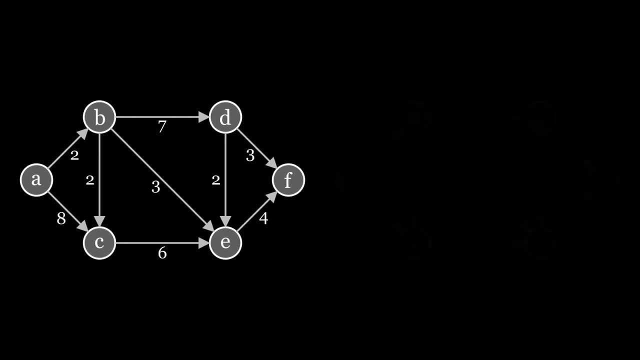 residual graph. In this way, we can undo the choice of bad paths which do not lead to a maximum flow. So let's go back to the first step. Let's choose the same path as before, but this time we add backward edges with 0 capacity. 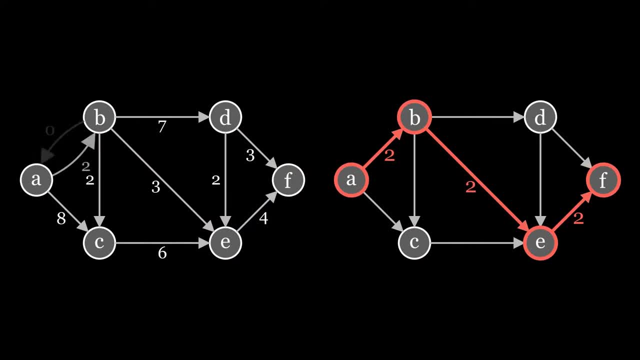 before computing the residual graph, We add backward edges also in the flow graph on the right. By doing so, we are highlighting the fact that the flow can also move back through each edge. Now we can compute the residual graph. Let's do the same with the second path. 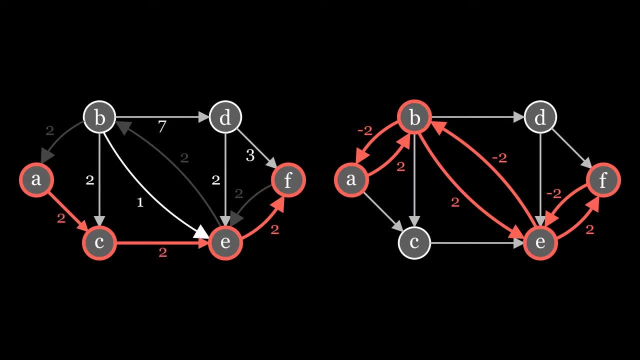 Once again, 2 is the bottleneck for the flow along this path. Let's add backward edges to both graphs. Now we compute the residual graph. Now we can see that there is a path that before was not available. The backward edge from E to B allow us to understand the flow of the path. 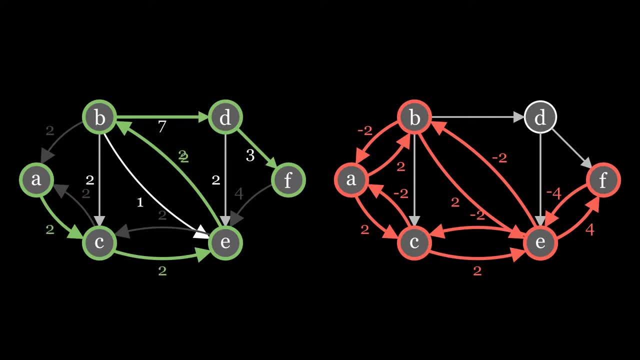 undo the bad choice that we made in the first step. We add this new flow to the previous one and add backward edges. Now we compute the residual graph. At this point there are no more paths available. the algorithm stops with a flow of 6.. 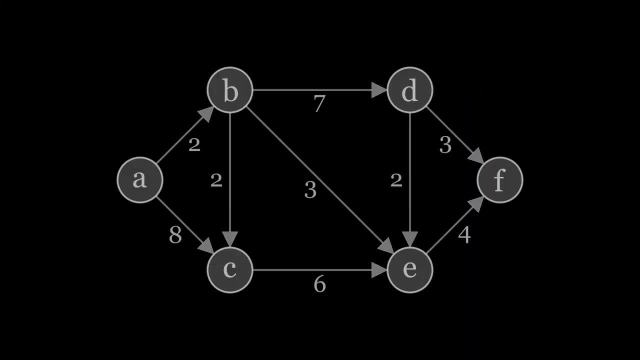 Is there a way to prove that 6 is the maximum flow possible? Let's introduce the idea of cutting a graph into two subsets, one containing the source and one containing the sink. The capacity of a cut is given by the sum of the capacities of the edges crossing the 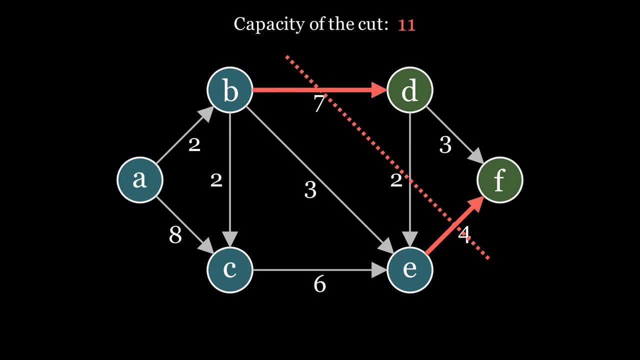 cut starting from the partition containing the source. It is possible to cut the graph in different ways. Let's see how it works In this context. we are interested in a minimum cut because of the max-flow-min-cut theorem that states that the maximum flow is equal to the minimum cut. 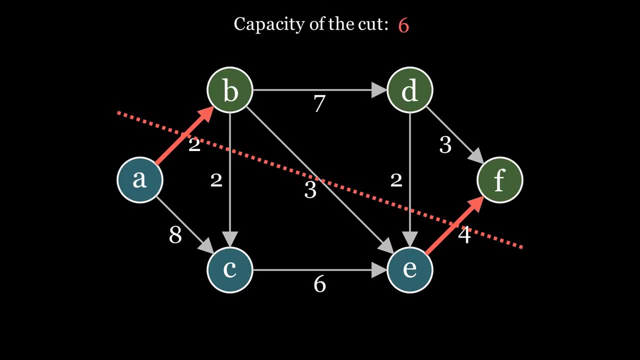 We can conclude that 6 is the maximum flow possible for this network. 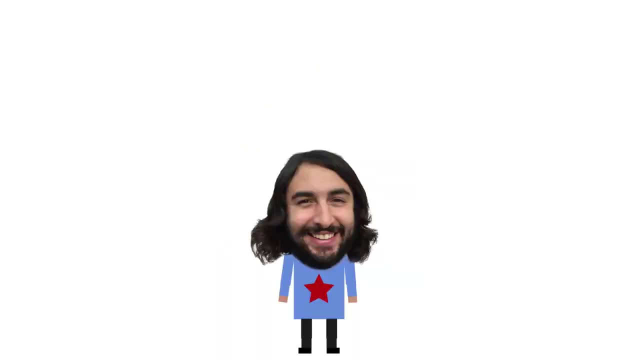 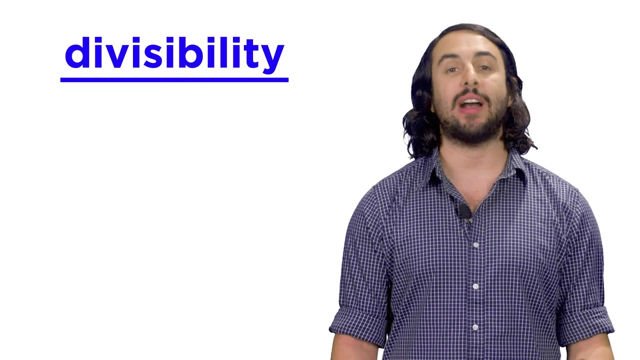 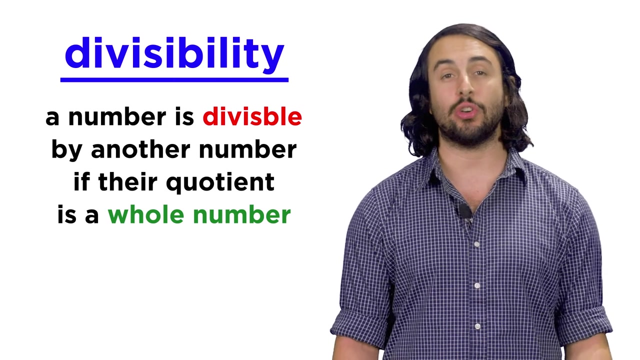 Hey, it's Professor Dave. let's talk about prime numbers. After learning about division, it's only natural to talk about the concept of divisibility. Numbers are only divisible by certain other numbers, which means that they can only be divided evenly in certain ways. 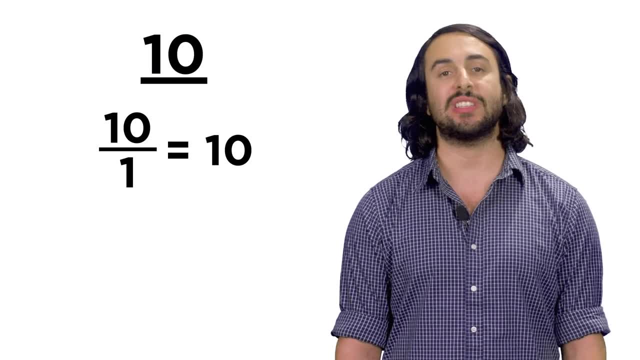 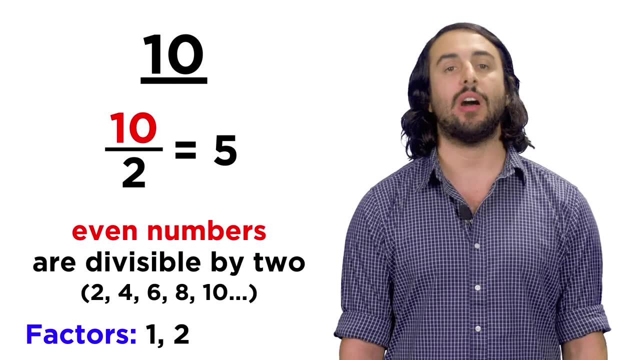 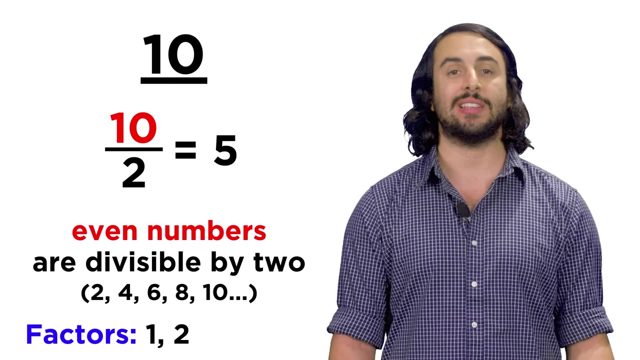 Take the number ten. Ten can be divided by one, which just gives ten. In this way, every number is divisible by one. Ten is also divisible by two, because it is an even number. Even numbers are the ones that are divisible by two, like two, four, six, eight and so.